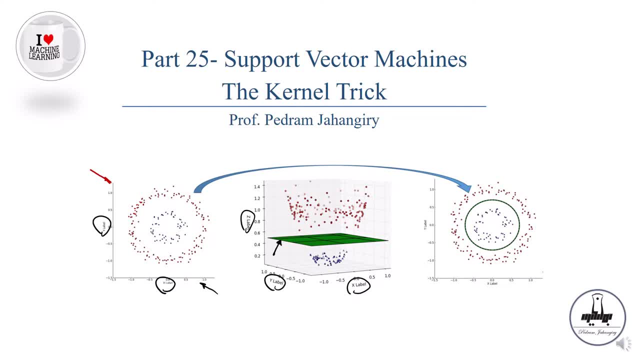 easily separable using this hyperplane, right, And then we're going to project it back to the two dimension again. So there's the steps involved. like this, we go to higher dimension and we find a hyperplane, we then translate it back to the lower dimension right and find this basically nonlinear decision boundary. So this is our nonlinear decision boundary, which is projected back to two dimension, right. So this idea is is going to work, But the problem is that it's going to be computationally. 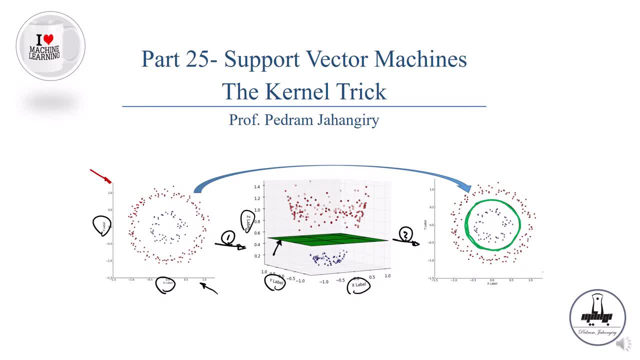 very expensive, right, especially when the dimension of the data set is very large and you have to go multiple dimensions higher to make the data linearly separable. right, and because of this cost of computations, we need to do a trick, and the trick that we use is called kernel trick, at the core of the kernel. 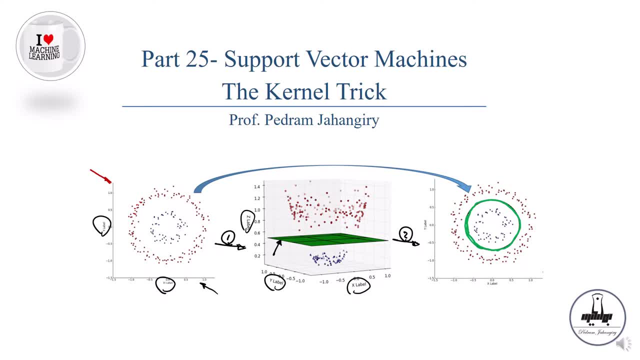 trick, we try to find a nonlinear decision boundary, but without going to higher dimension. we're going to bypass this step right. so using a kernel trick, we go directly from this step to this step: finding the nonlinear decision boundary. the term kernel can be thought as a similarity function between a pair. 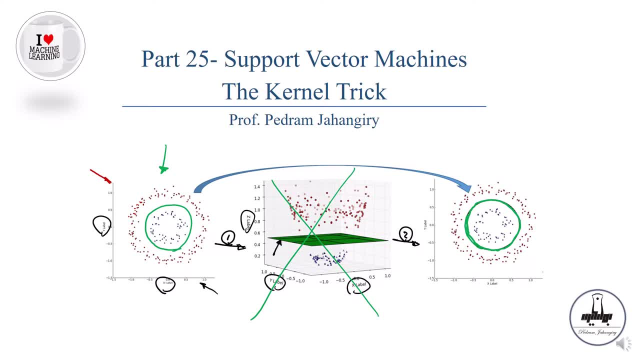 of samples. so, for example, we can think, depending on what functional form we use for the kernel function, we can come up with different methods to basically look at the distance between every pairs of observations and assign a number to them. right, and based on those numbers we can. 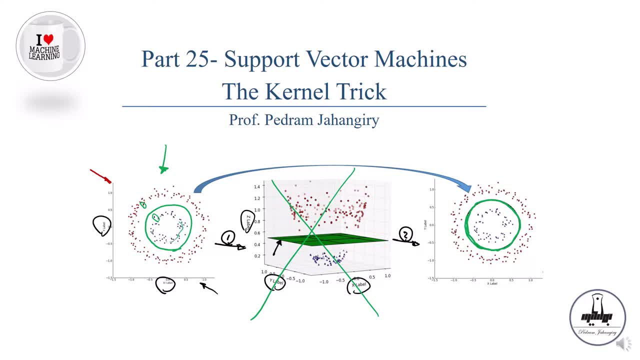 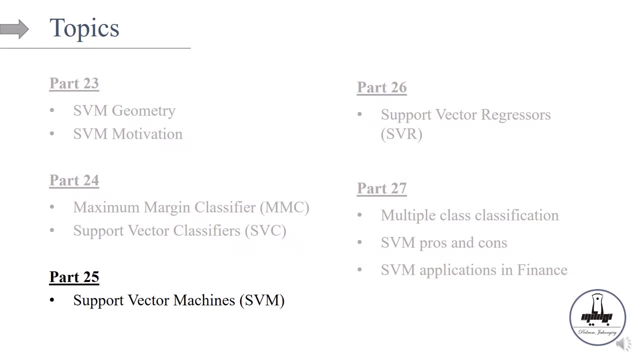 say: okay, for example, these blue lines are close to each other and so make a decision boundary. let's make a decision boundary like this: okay, now let's see what is inside that kernel trick and how how it's doing the job. in the previous part, episode 23 and 24, we covered some basic definitions of SVM and we 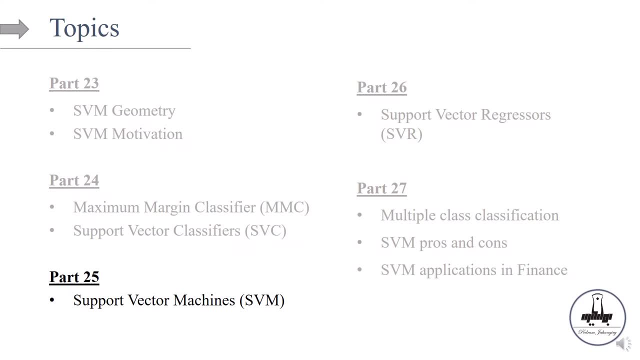 basically explained what is the difference between the hard margin and soft margin. we said why we need to go beyond the hard margin, and so we extend the idea of hard margin to the soft margin. in this episode, part 25, we're going to explain why soft margin. 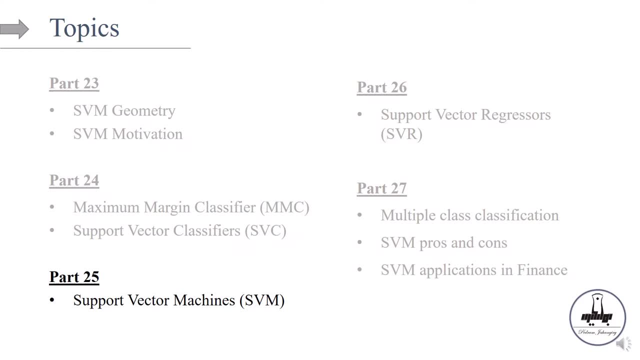 alone is not enough sometimes and we have to extend the idea of soft margin with something else. so we're gonna add the concept of kernel trick to the soft margin. so the combination of kernel trick plus soft margin, so soft margin plus kernel trick, is what we call SVM, support vector machines and in general, 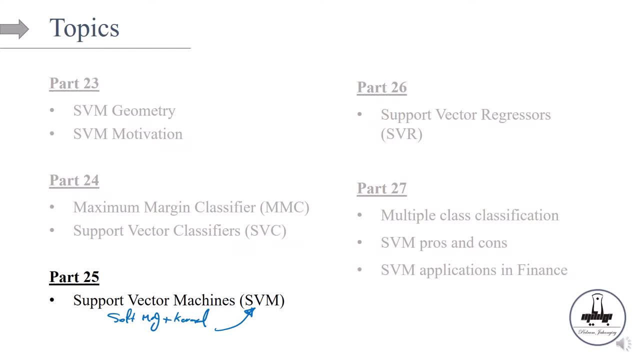 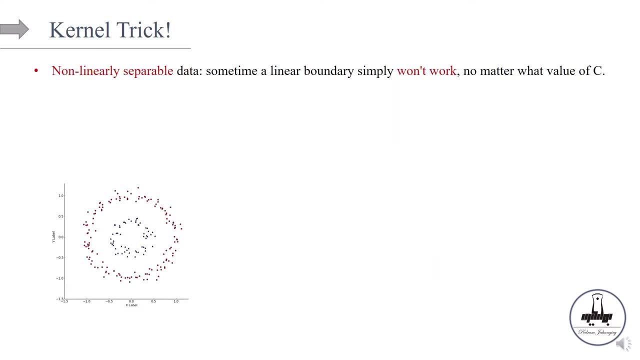 for all these classification problems. we're going to call it SVM support vector machines. what is the kernel trick? well, we know, when we have non-linearly separable data, a linear boundary simply does not work. it won't work, no matter what value you use for the the. 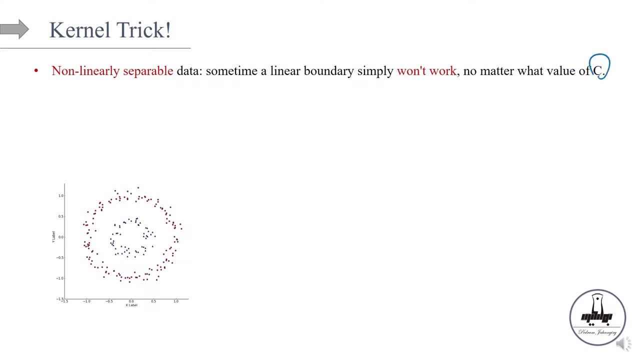 regularization parameter c. remember this. c was something that was controlling the bias variance trade-off in our SVC models, right, the the support vector classifiers, where we were using the soft margin. now here, just think of this case that imagine, this is your hyperplane and this is your margin, no matter how you change the value of c, for example, if you decrease c, the margin is. 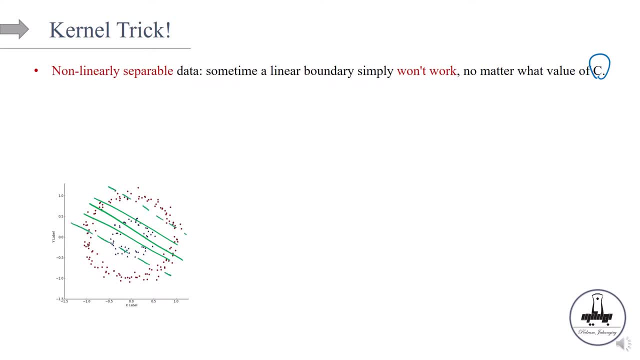 going to get wider and wider, but whatever you do with that number, it's not going to help in terms of getting a better model, because there is no way that we can use a linear separable model to get a better model, because there is no way that we can use a linear separable model. 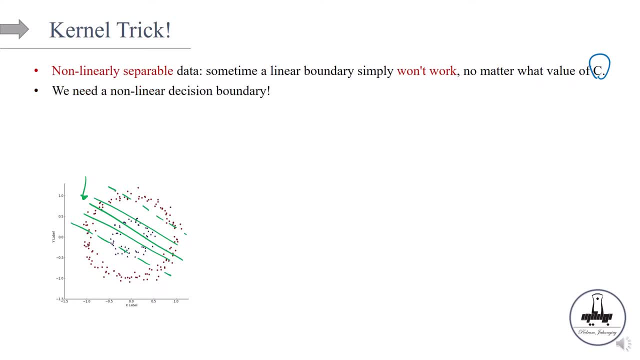 creating hyperplane to do the job for us, so we need a non-linear decision boundary for that. one way is to map to higher dimension space, finding the hyperplane and projecting it back to the lower dimensional space, and we know that this can be computationally difficult. so how do we go to higher? 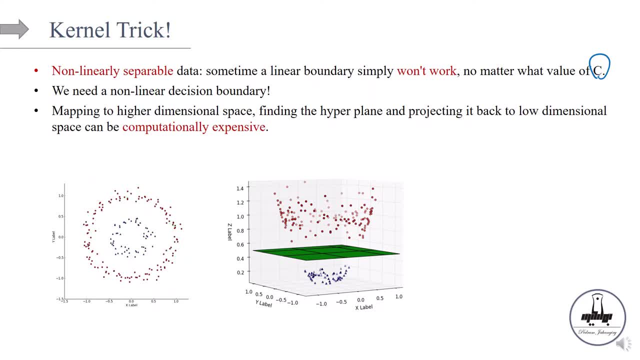 dimensional space, for example. so here we have two variables right, x and y. so we can define z as a function of the non-linear decision boundary. so we can define z as a function of the non-linear decision boundary. so we can define z as a function of the non-linear decision boundary. so we can define: 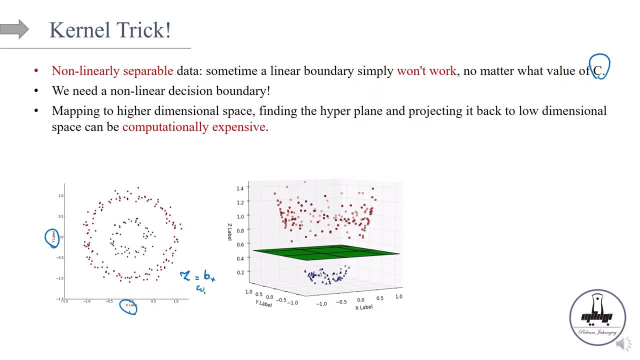 some. for example, we have b plus w1, x plus w2, y plus w3, x, squared plus w4, y, squared plus something right if we think of z as a transformation like this for x and y, so it's going to when we go to three. 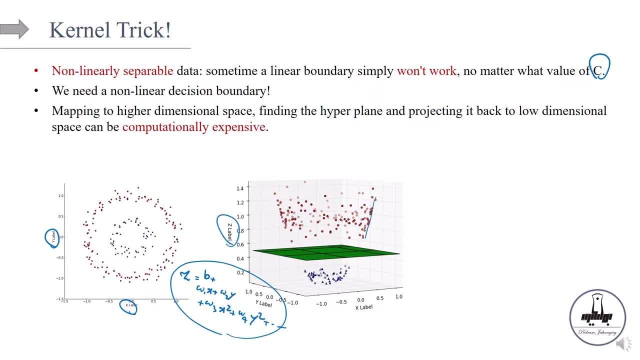 dimension, the shape is going to be something like this. right, it's going to be something like this, and then, as you can see in this new three dimension, it's easily separable using this hyperplane. finally, we can project it back and find our non-linear decision boundary okay. so the kernel trick is doing this job without going. 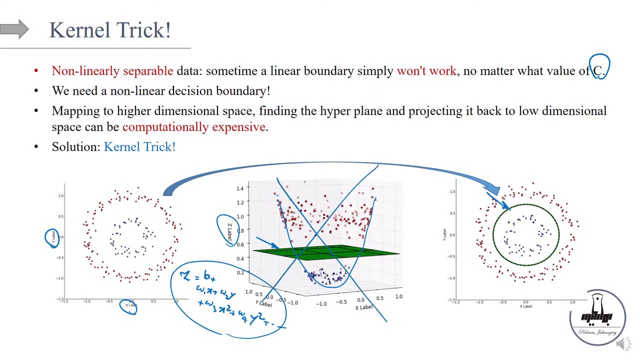 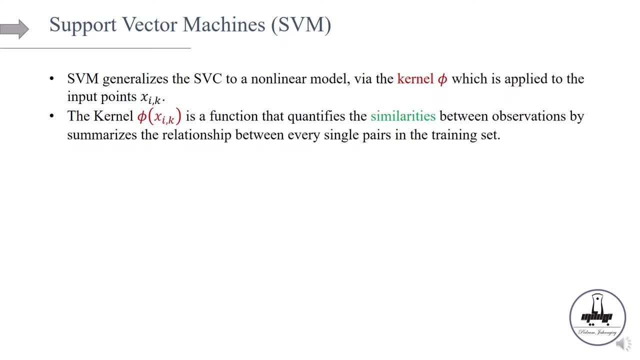 to the higher dimension. so it's going to help us a lot in terms of speeding up the computation. now let's look at the optimization problem in svm. so svm generalizes the svc to a non-linear model. now let's look at the optimization problem in svm. so svm generalizes the svc to a non-linear model. 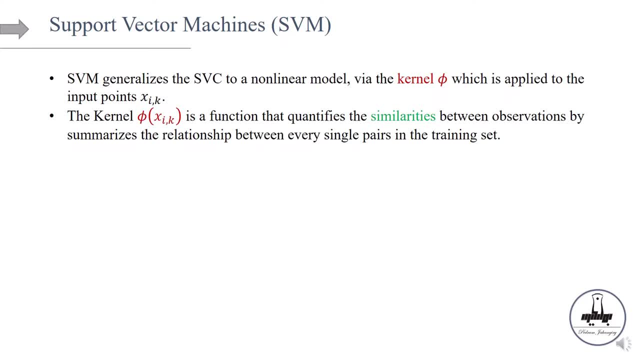 we are using the kernel function phi, which is applied to every point in the data set, right? so the kernel phi is a function that quantifies the similarity. so this is really important. it quantifies the similarities between observations by summarizing the relationship between every single pair in the train set. okay, so it's going. 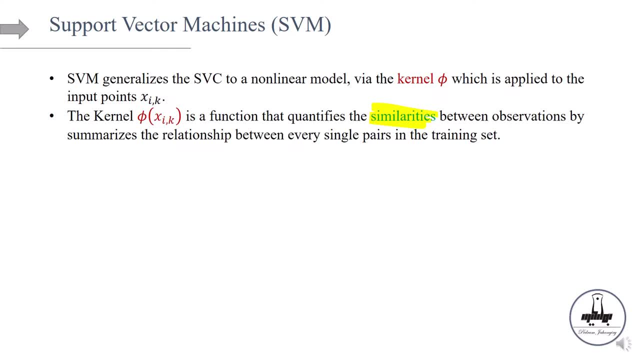 to look at in each pair in the in the train set and assign a number to that pair of observation and that number is representation of the similarity between those observations, right, and then we can write the optimization problem like this. so this is pretty much the same as the. 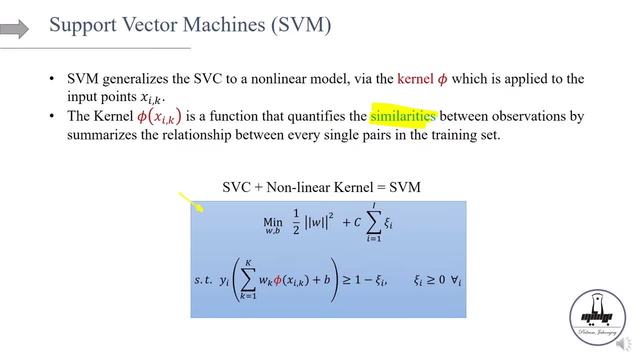 svc is the soft margin optimization problem right, and the only difference is this part: here, instead of using a linear combination of weights versus x's, we're going to use a function phi of x's and y, right? so the idea is that we're using a soft margin, right, we are giving some 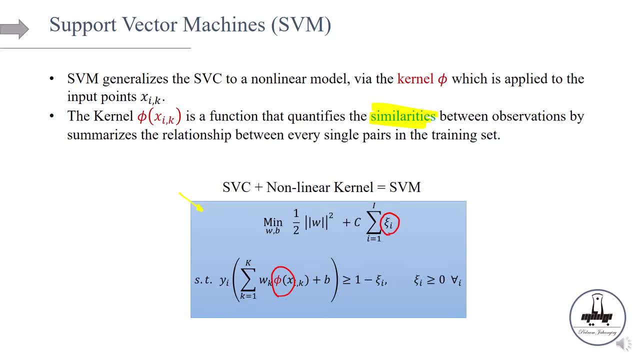 slags to the observations, to be on the wrong side of the margin, and we're going to penalize those slags, the sum of those slags. so by this penalization we are regularizing, we are making the balance between bias, trade-off, and so here, this is our constraint, the same story. 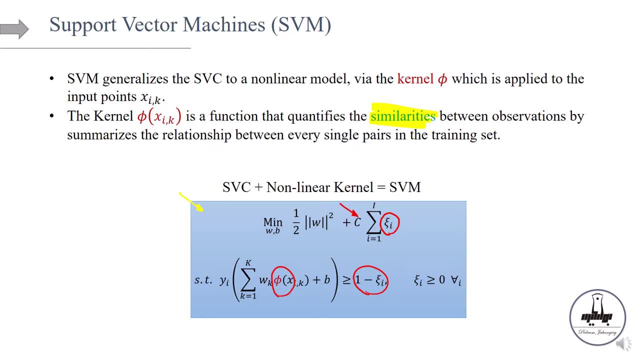 we are giving some slags to the observations inside the margin and the only difference is this part: how we define the relationship between the between the observations in the train set, right, okay. so let's clear some terminology first, if we have svc- we talked about the soft margin- okay, so we can think of svc- 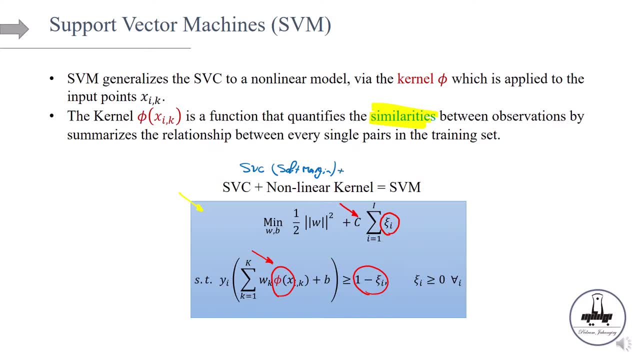 as soft margin plus linear kernel. right, so you can think of it: soft margin plus linear kernel. this is what we use as the terminology. we use support vector classifiers. if we use hard margin, hard margin, we call it mmc- maximum margin classifier. so there are three terms that i want. 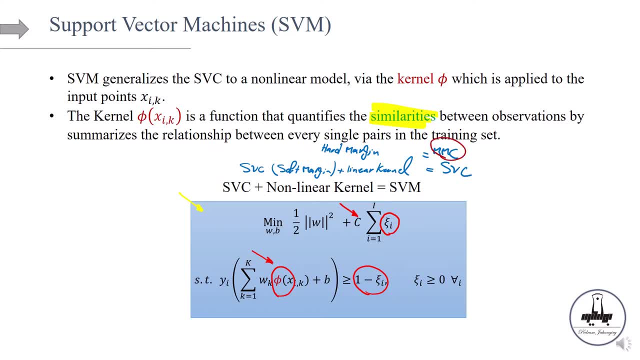 you to be aware of. one is mmc, that's this hard margin. the other one is svc, when we use a soft margin, and finally svm: it's a combination of soft margin when we're using the soft margin classifier using a non-linear kernel. okay, so from now on we are going to use the term svm in a general version. 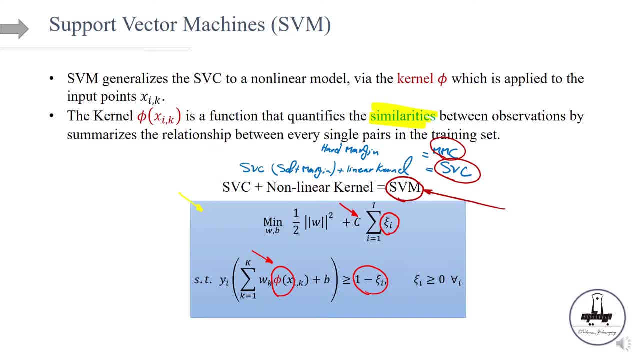 so support vector machines, and we can think of svc and mmc as a subset of svm, depending on what functional form we use for the, the, for the kernel function and if you're giving the model a slack or not. okay, so, in short, support vector machines, use something called kernel functions to systematically. 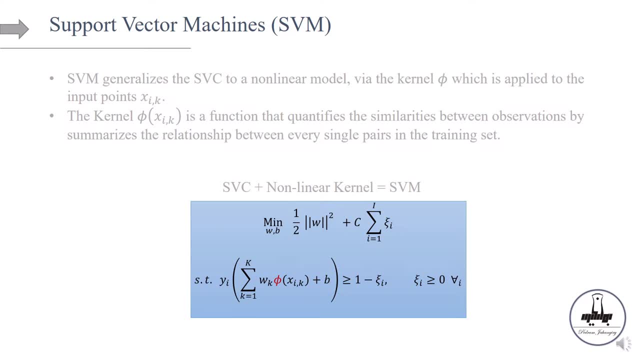 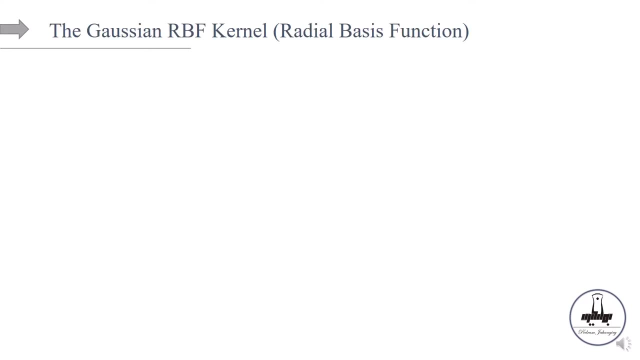 find svcs in higher dimensions without going to that higher dimension. so this is a fascinating idea. now let's talk about some of these kernel functions. there are many different kernels available and one of the most famous one is called radial basis function. radial kernel is one of the most famous ones that the main part of it is coming from, the multivariate. 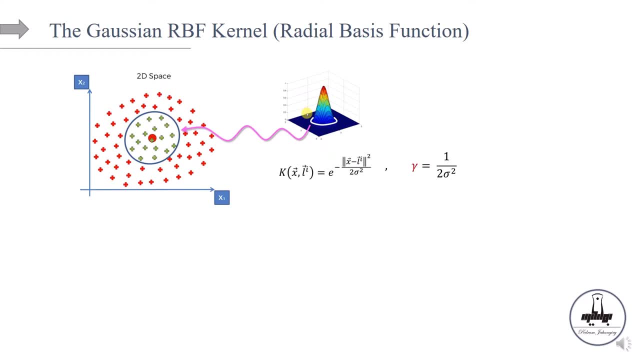 distribution. so let's look at an example. so imagine, this is our data set in two dimension, x1 and x2, and we have two classes, red and green- and, as you can see this, this problem is non-linearly separable, right? so we have to use our kernel trick. 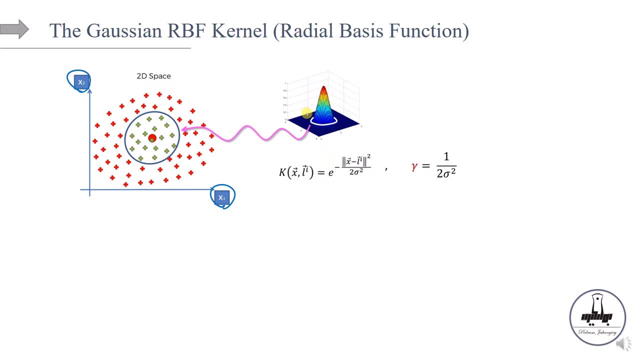 so how does the kernel do the job? remember, the idea of the kernel was to assign a number which represent the similarity to any pairs of the um data in the train set right. so we're going to look at each of the observations. let's say this one or 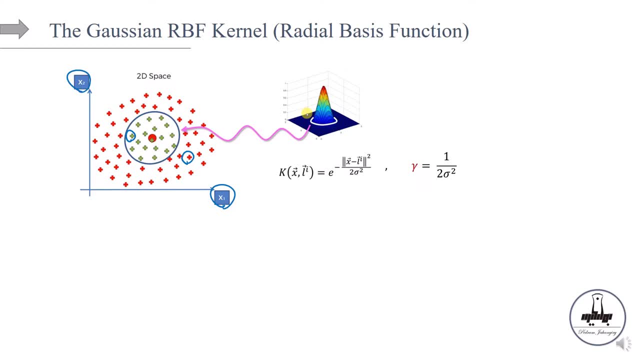 this one and pair it to another observation, which we call it landmark. so let's pair it to landmark and this landmark is what it's shown in in red here, right? so this is our landmark point, right, and the kernel is going to find the similarity between any each observations from that landmark. 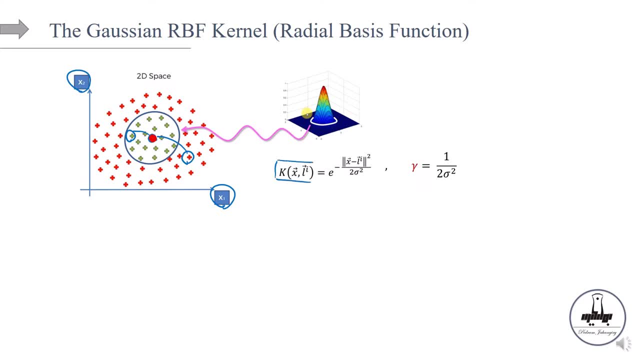 so what is the functional form? this is a functional form. we're going to quantify the similarity between any x and the point that we call it landmark. so where we put the landmark and what the how we decide. what is this landmark? this is another optimization problem itself, but let's take it. 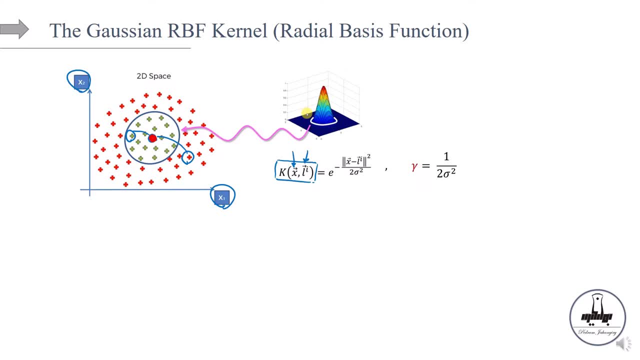 as given now, and calculate the distance, the similarity between any observation in the train set from that landmark. so here is a functional form. it's e to the power of minus, the distance of x minus lambda to the power of two, this divided by two sigma squared. so this is coming from gaussian. 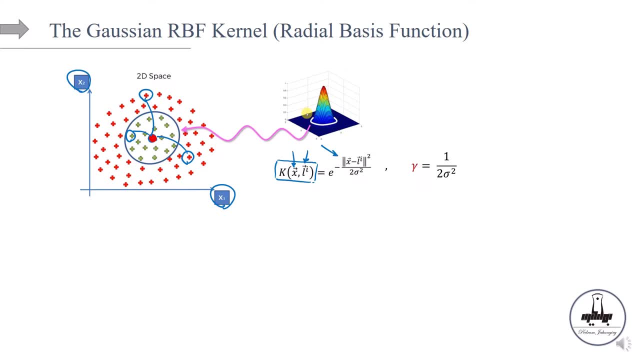 distribution, right. so we are familiar with this functional form already. and now let's define the parameter gamma well, as one divided by two sigma squared. so basically, gamma is inversely related to the variance, uh, of the, the, the gaussian distribution that we are looking into right now. let's take two points. let's say this point: 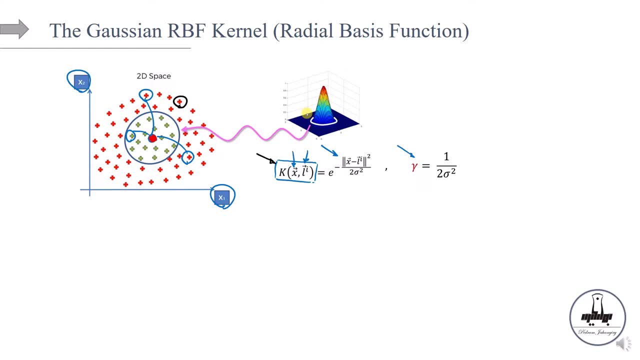 and see what is the value of k for that. okay, so if, if that point is far from the land mark, we know that the numerator is going to be large, so it's a positive number. e to the power of minus, a large number is going to be smaller. so here we get a small value for k, and if the 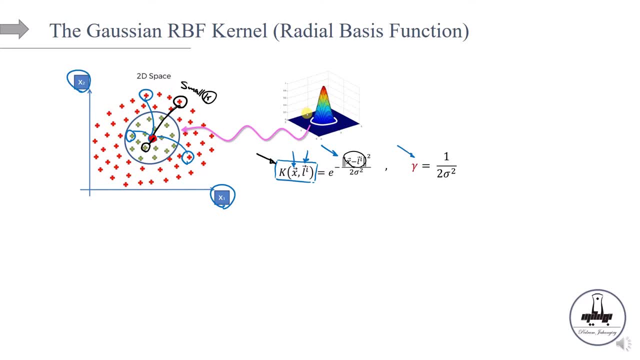 if the observation is very close to the landmark. so we get a large value for k. all right, so k remember that is that. uh, our kernel trick right at the kernel function, right, so, as we can see then, we have bunch of observations in the train set that we 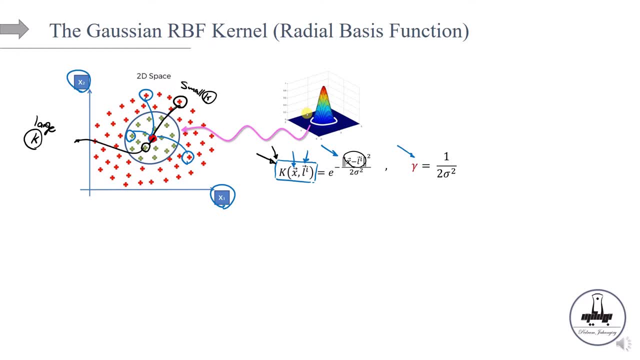 assign a number to them, so a small number or a large number, and based on those small or large number, you're going to classify them into two groups, because we are going to come up with that non, no, non-linear boundary. okay, now let's talk about gamma. we know that gamma is inversely. 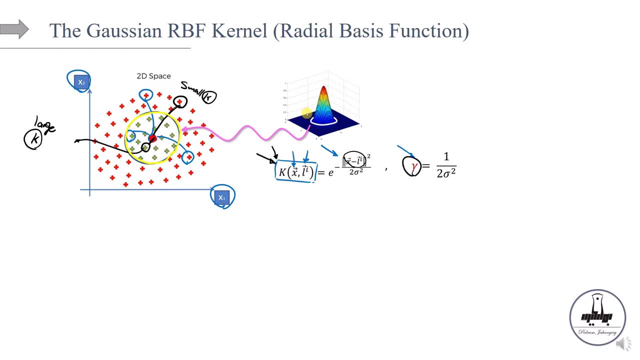 related to the variance and what will happen if we increase the gamma, right? so when gamma is large, i e, so gamma is large, i e. sigma is a small, so we are going to reach out to closer points, right, because this variance is going to be smaller. right, so we're going to reach out to closer and closer points. so in two dimensions, something like. 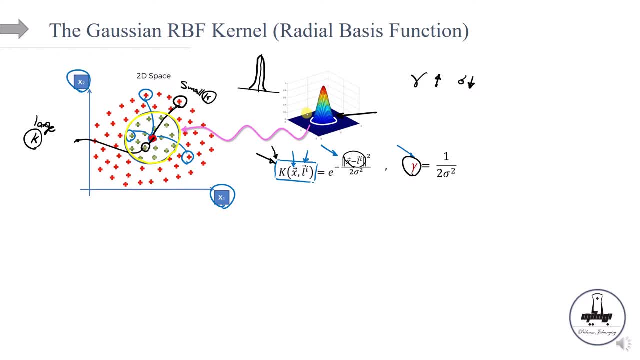 this right. so this is gamma. gamma is going to large, sigma small, versus gamma is going to small, sigma large- right. so when gamma is large, we reach out to closer points, and if gamma is small, we reach out to further points. right, and so we reach out to further points by. 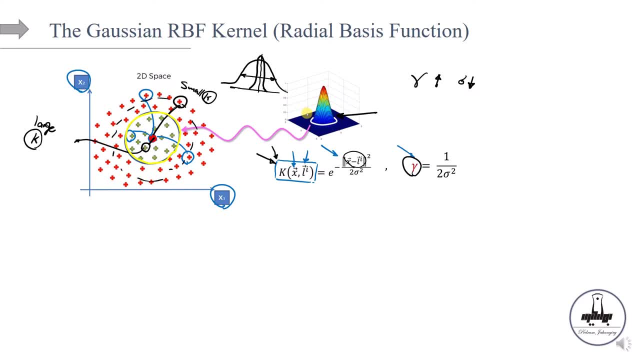 this decision boundary, so let's see how it's going to look like in an example. so here we have a two-class classification problem and, as you can see, the data is clearly nonlinearly separable. right? so we have one purple observation here and not a purple observation here. a bunch of purples here. 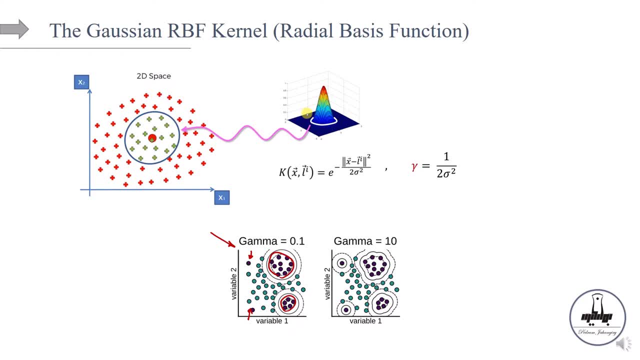 and bunch of purples here and the rest of it in the screen, right? so we know that we have to use the Cornell trick and the RBF is a good suggestion here there because of these local clouds of the data. right then, if gamma is a small, 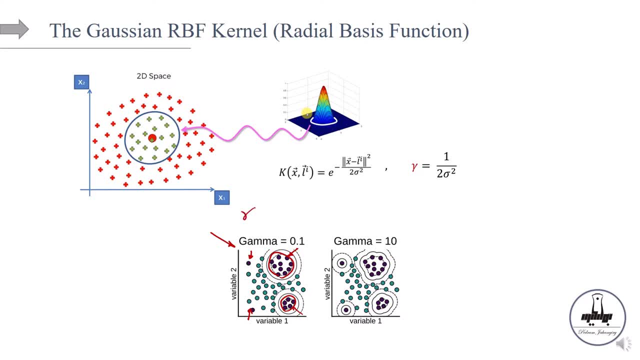 so if gamma is a small, we know that Sigma is large, so we are reaching out to further points around that land landmark, right? so if gamma? so let's say if gamma is point one, we are going to end up with two landmarks, and these are going to be: 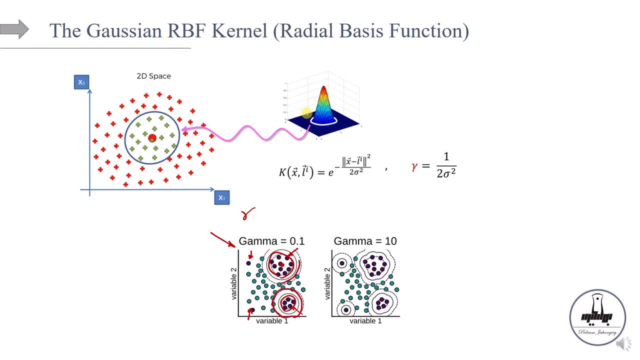 our decision boundaries, right, basically one, one area here and one area here, right, if the gamma is large. so we will try to reach out to closer neighborhoods. right, you are trying to reach out to the, let's say, more local neighborhoods, and then it is done by, in this example, by finding four. 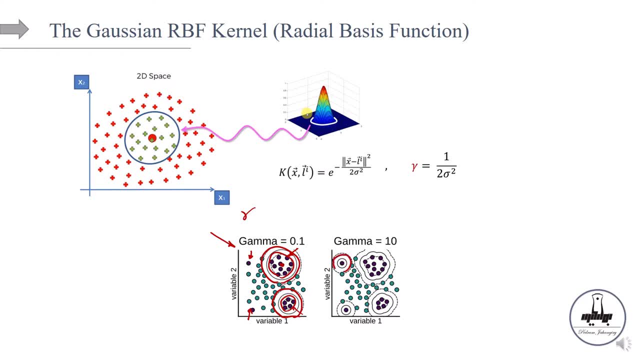 landmarks and, at the end of the day, we're gonna end up with this decision boundaries right. so, as you can see the, when you're increasing gamma from point one to ten, you're making this model more complex. but more complex we mean that it's going to have it smaller bias, but on the other hand, the model variance is going to be. 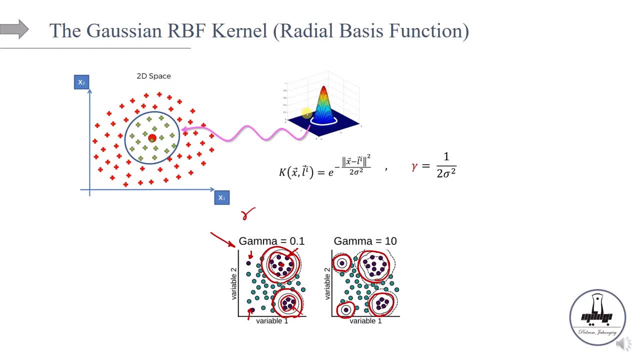 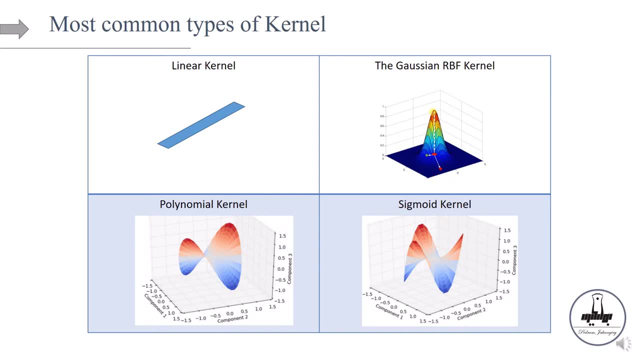 larger. we're going to talk about gamma as a tuning hyper parameter in the next slide. so what other type of kernels functions do we use most of the time? so another one is linear kernels. so we are all familiar with this linear kernel. at the end of the day, it's going to look like our know separating hyperplane and 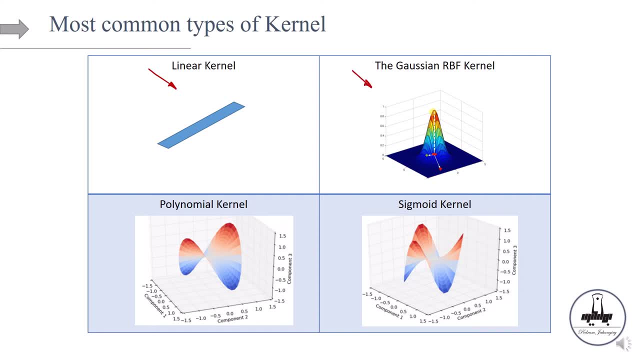 the one that you just invested in is the linear kernel, and that's where we're going to- is the Gaussian RBF kernel, the another one is polynomial kernel and, finally, we're going to work with sigmoid kernel. so all these kernels are going to help us to just remain in the same dimension of the feature space, without going to. 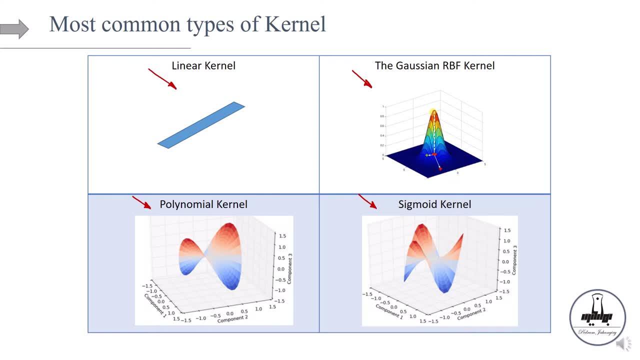 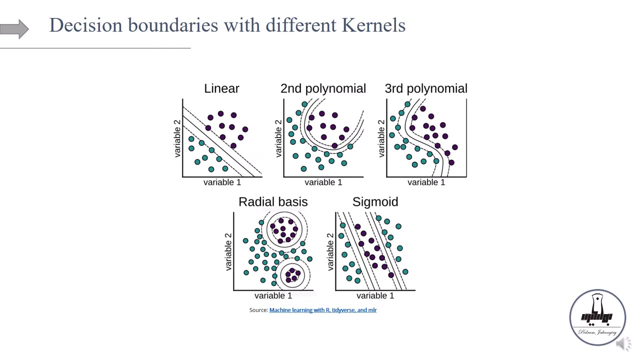 higher dimension and find the separating hyperplane. so it's going to help us to reduce the computation a lot by avoiding to go to higher dimensions. let's look at some decision boundaries with different kernels. okay, so imagine we have seen all these examples. it is to class classification, you know class green. 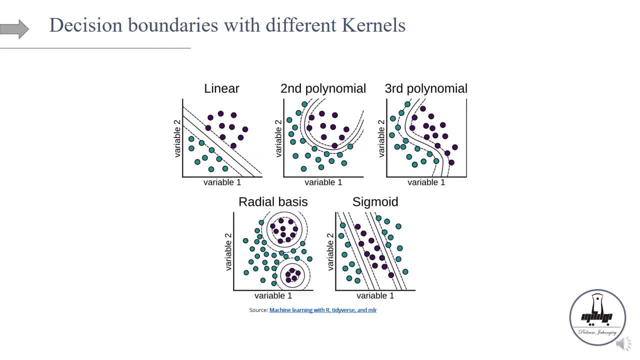 versus class dark purple. okay, in the first one, we are using a linear kernel, right, so this is SVM using a linear kernel. you can think of it as SVC support vector classifier, and so, if the data is well behaved, the linear kernel is going to do a decent job, as it does here, and in the middle we can look at: 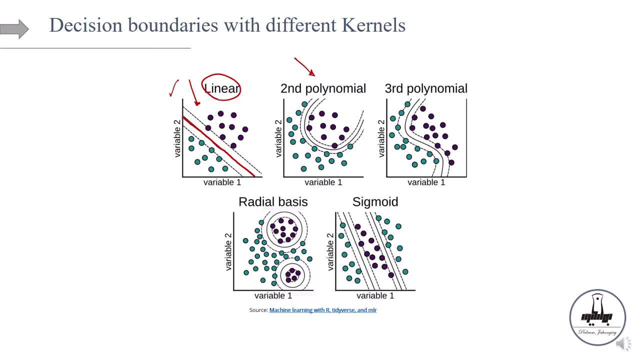 the SVM using a second-degree polynomial kernel, right so- and as you can see, this is going to enable us to bend the decision boundary like this: and if we use a higher dimension of polynomial, the decision boundary is going to become something like this: right, and then, on the left button, we have our RFP radial. 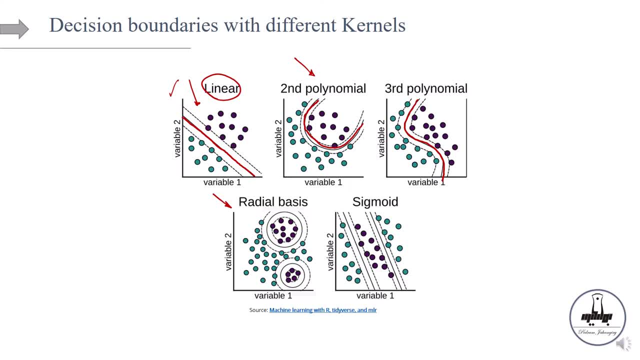 basis. so this is as we saw. it's using Gaussian distribution, basically looking at these more kind of local, the cloud of data. and then, finally, we can look at the sigmoid kernel function which is going to separate data like this for us, right, if you're interested in the details of the formulas for sigmoid and 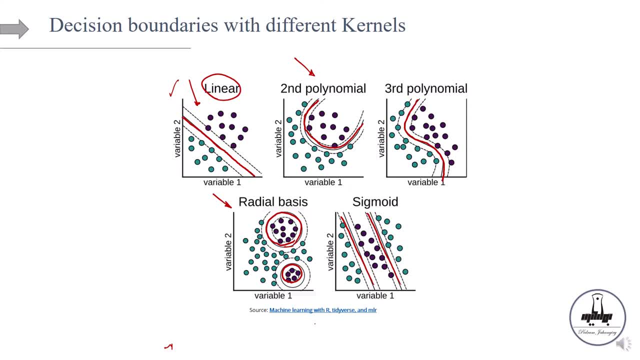 polynomial kernels. you can read the documentation in the scikit-learn package or basically look at the documentation in machine learning with R. okay, and basically if you google it, you will find the tons of extra information for all these kernels. okay, but for this short video we're going to try to avoid. 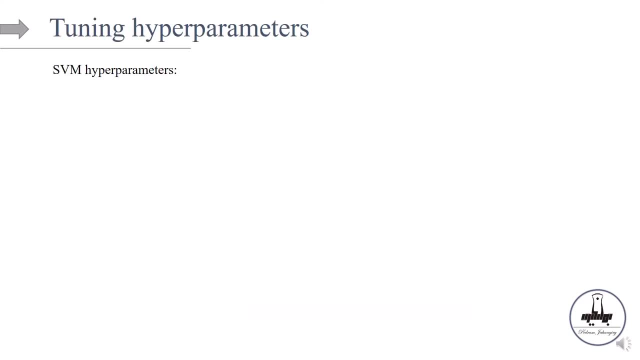 those technical things. okay, so how do we tune the hyper parameters in SVM? right, so what are the hyper parameters that we are mostly interested in? SVM is the first one. the main one is C: the cost of making errors right and cost of misclassification. this controls the bias variance trade-off. so we discussed this. 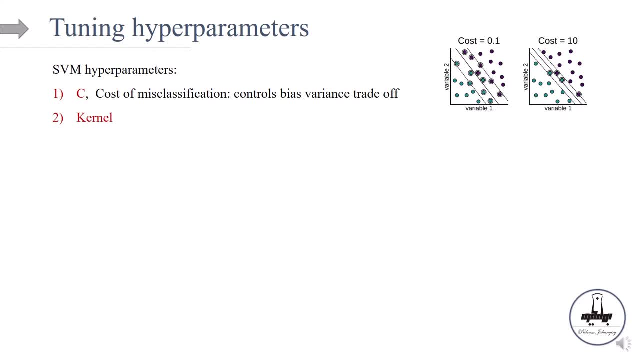 one earlier, that if the C is a small, let me use red pen- if C is a small, we are going to have wider margin. if C is large, we're going to have a narrow margin. the second one is the kernel function itself. so we know that we can use, for example, polynomial. 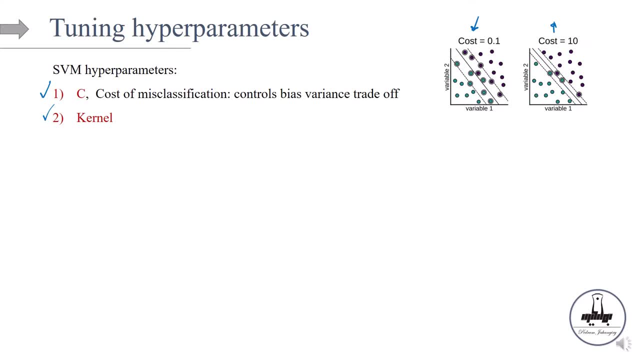 RBF, linear kernel and sigmoid and etc. the third one is gamma. actually, gamma is used only when the kernel is RBF, and RBF kernel is one of the most commonly used ones. right gamma controls how far the kernel is from the kernel to the kernel. right gamma controls how far the kernel is from the kernel to the kernel and the 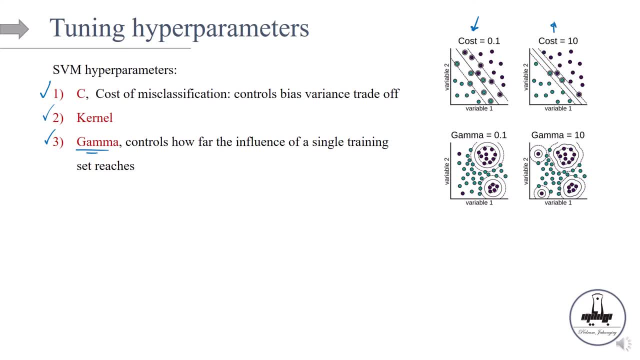 how far the, how far the influence of a single training set reaches, right. so when gamma is a small, we are reaching out to further observations. when gamma is large, we watch and you know two closer observations, right, okay, how can we tune these hyper parameters? we can use a great searched cross-validation method to tune the. 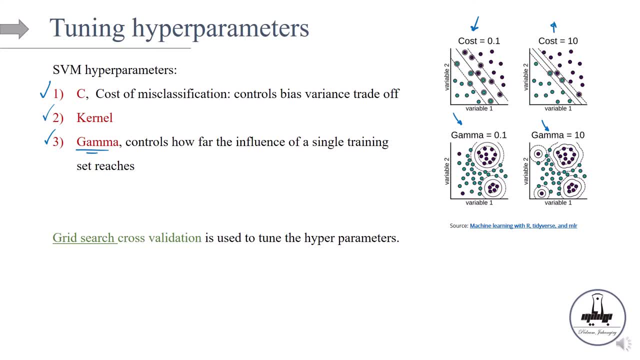 hyper parameter, right. so the grid search, cross validations is a combination of great search and the cross-validation, as the name suggests, right. so the idea is that finding the right parameters and testing and other things together it parameters like c, gamma and etc. is is a little tricky, right, but we can do. we can just try a. 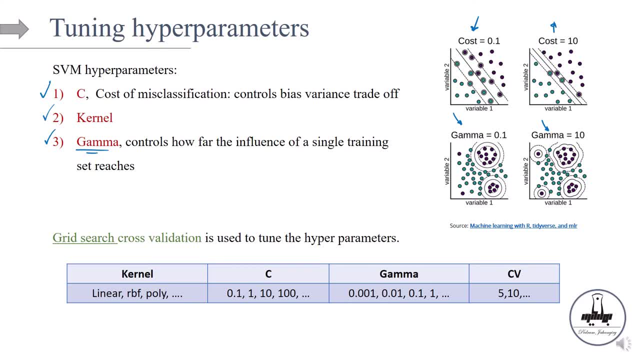 bunch of combinations and see what works best, right? so, for example, we have these values for kernel, these options for kernel. we try out these values for c, we try these values for gamma, and we can use either five-fold cross-validation or tenfold cross-validation or any other number. 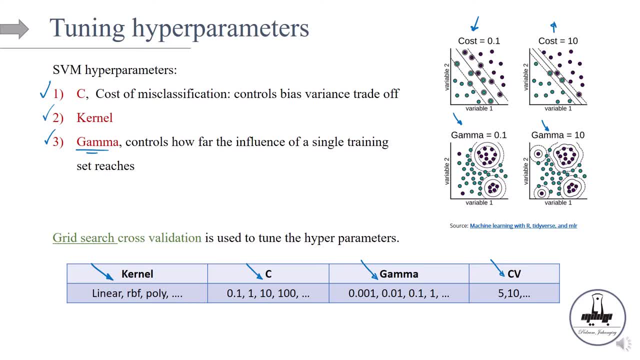 so the idea of creating a grid of parameters and just trying out all the possible combination is called grid search, and this method is very common and that scikit-learn has this functionality built in with grid search cv, grid search cross-validation. so just remember: grid search cross-validation may seems interesting, but it is computationally very expensive. 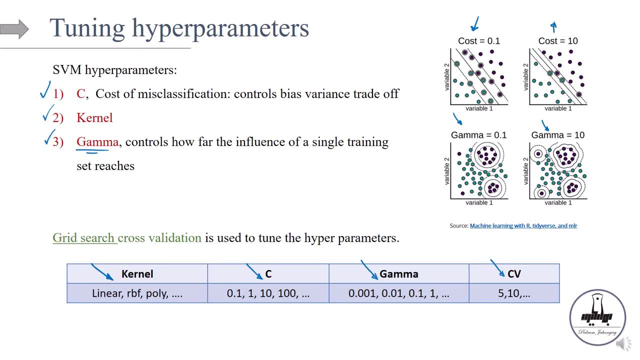 and it's time consuming if the data set is large, right? so in this example, let's say we have four different and three different kernels, uh, one, two, three, four, four different c's and four different gamma, and let's use only five-fold cross-validation. so we have three by four by four. 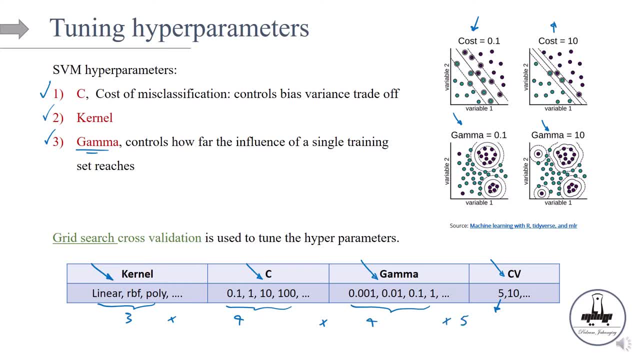 by five or 240 different iterations that the computer needs to go over the entire data set. now let's imagine that the data set has millions of records, so 240 times of all those calculations of uh multiplying million, right? so the? and there's another point of grid search, cross-validation as 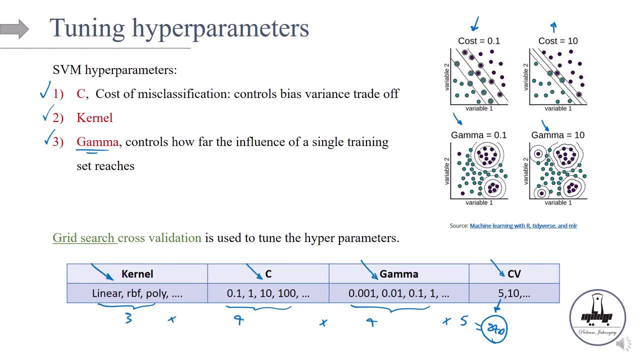 well, and the idea is that look at the hyper parameters. you know c is a continue, it can be a continuous, random hyper parameter. kernel is discrete, so we have some discrete choices, and gamma is also continuous, right. so we cannot simply use methods like gradient descent, or we cannot use 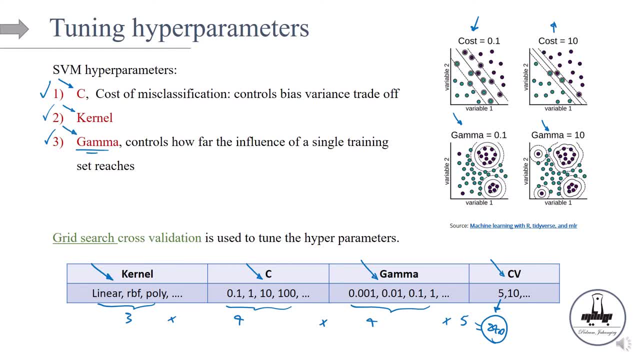 simply use method like no elbow method. so we have to just try and error different combinations. but we have to try and figure out which one is the best. right we again. it's going to be computationally very expensive. how do i know that these are the better numbers right? so the overall. i want you. 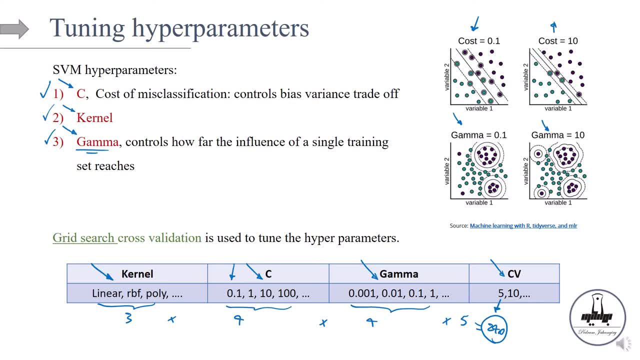 to think of this grid search as in as an- i well, maybe ideal method for tuning the hyper parameter, but that's not necessarily the best one out there, right so? and there's a good chance that sometimes, when you're doing the grid search cross-validation, you're not getting a better performance to 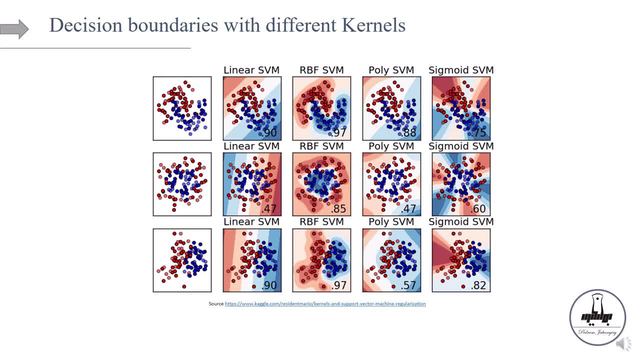 compared to the plain vanilla version of the svm. so let's talk about the data sets first. so imagine we have two class classification. basically, the classes are red and blue, the plot shows the training points in solid colors and testing points in semi-transparent. so this is it. this is a train point, this is a test point, right, this is a. 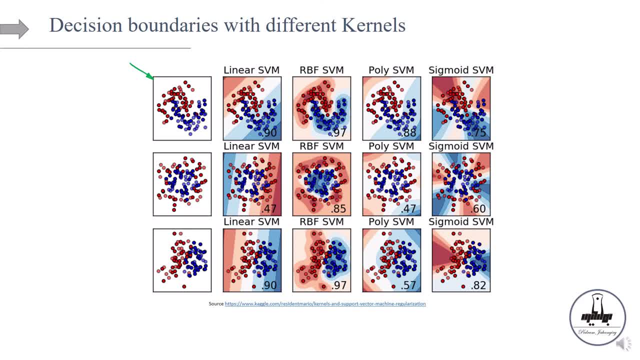 train observation. this is a test observation, so overall, they're going to be very similar to the data set. so we're going to be using different types of data set here. so we're going to be using different types of data set here. so what are the colors? so let's talk about the data sets first. so 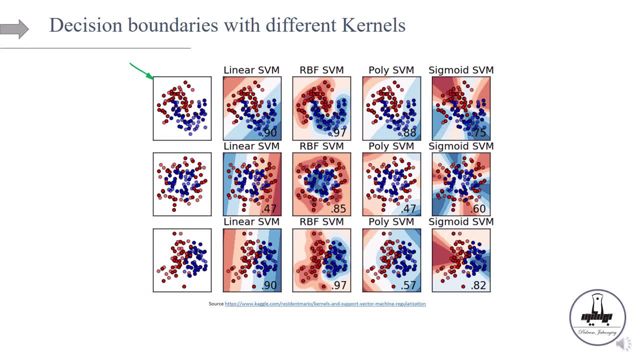 we're going to be using different types of data set here. so what are the colors? so we're going to be two classes right, red and blue- and then we're going to use different kernels and apply svm and see which one is going to perform better. so the metric that we're using is is accuracy. 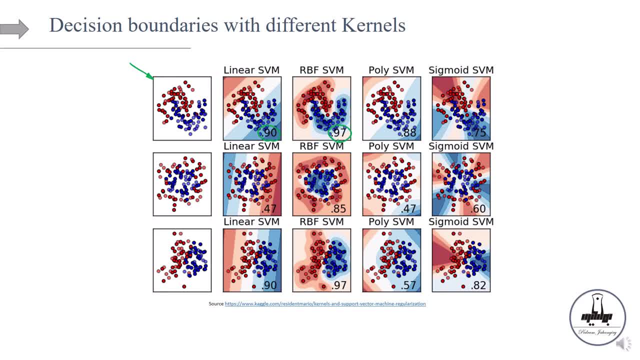 so the numbers on the bottom right are the accuracies, and now with that let's compare these different kernels using uh applying to the different types of data sets. right, so starting with this kind of moon shape data set, because you're, it's kind of two moons inside. 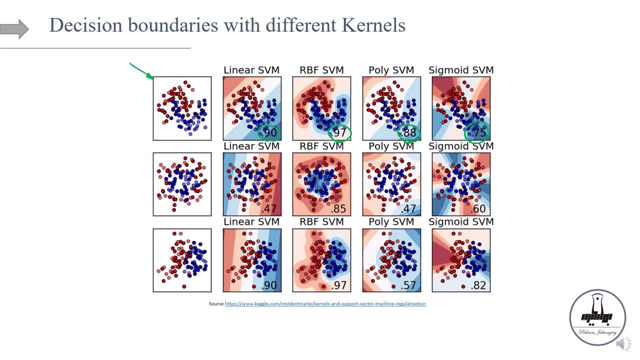 each other, right? so if you use a linear svm, so let me use another color. let's use yellow if you use linear svm, so we get something like this: this is going to be our separating hyperplane, right? and the idea of these colors is that the solid areas, the solid shaded areas, are the points that 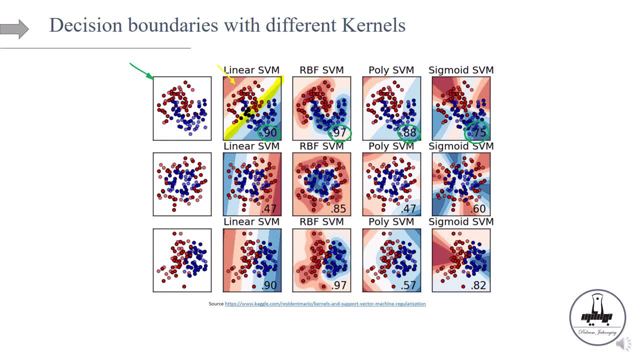 classification is more accurate and the the more transparence they get your the model is going to allow for more misclassifications, right? so here, at the bottom, right here, we're going to have a linear model, and the linear model is going to do a good job, you know, and the accuracy is 90. 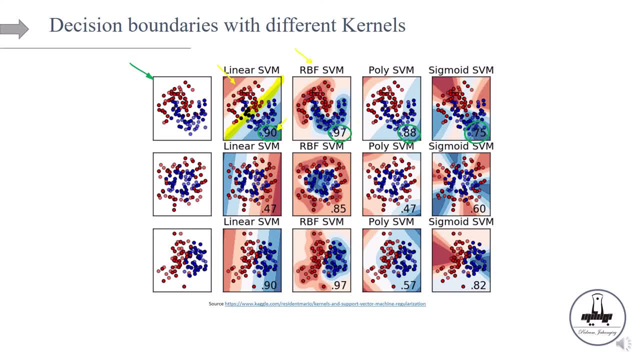 then if you use the rbf svm, the rbf svm actually is going to is able to do the perfect job. right, because it's cat, it's going to capture these local neighborhoods very beautifully. right, then we can do polynomial svm. with polynomial svm, the accuracy is 88 percent, and with sigmoid. 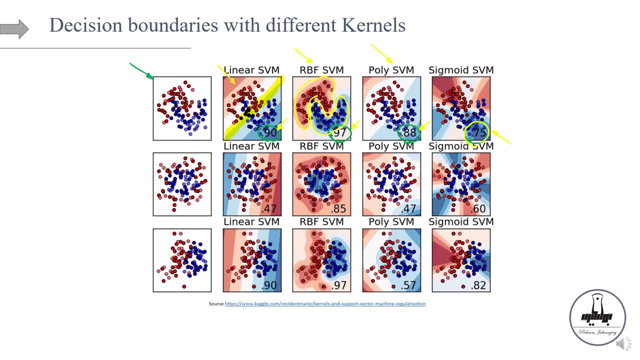 svm. the accuracy is only 75 percent, right? so the winner in the first data set is rbf. so let's, let's write down the veneer here, so rbf, rbf, svm. right now for the second data set. as you can see, this data set is clearly non-linearly separable. so we have, we have some idea that, a linear classifier. 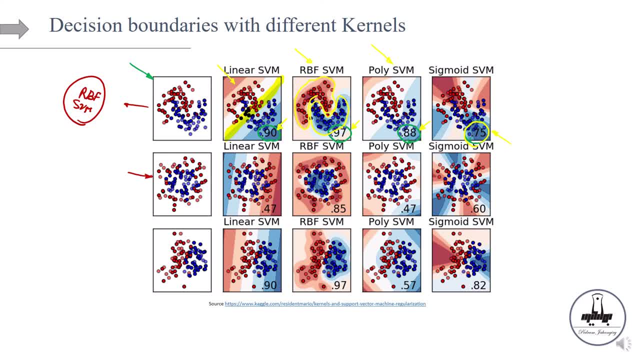 a linear svm should not do a good job and, as you can get, as you can see the, the accuracy is only 47 percent. so, not surprisingly, we know that any kind of linear is not able to do a good job here. and not surprisingly, this data set is designed for for rbf svm, so it's going to do a good job. 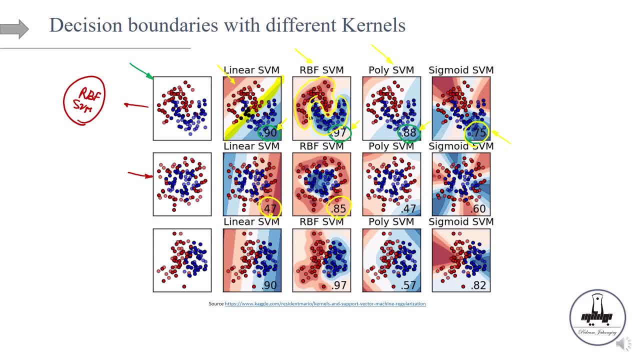 with accuracy of 85 percent. and, by the way, guys, these accuracies are the accuracy in the test set right. so these are the numbers that you're interested. if you use polynomial svm, the accuracy is 47 percent and for the sigmoid the accuracy is only 60. so again, the winner here is rbf. 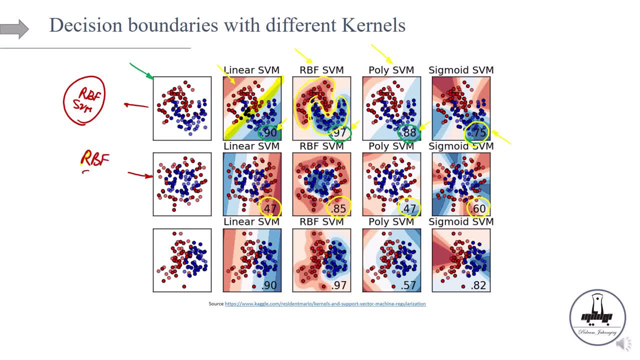 yeah, so let me write it with red: rbf: svm. look at the data that it's relatively linearly separable, so we can visually see that. okay, if you use a linear svm, it should do a good job, and actually that's the case, right? so look at the 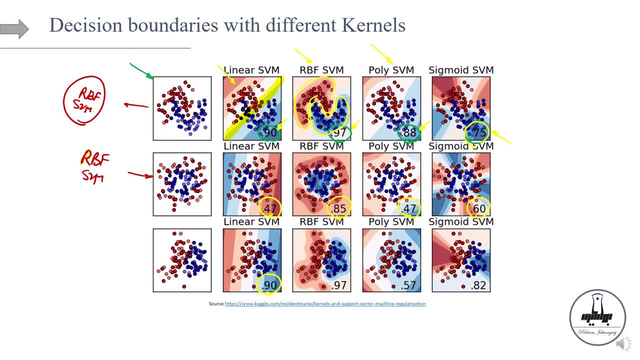 accuracy in the test set. for linear svm it's 90 percent, for rbf it's 97 percent and for polynomial is only 57 percent. sigmoid also, that is 82 percent. so so in this case we can say, surprisingly, rbf right, because the data was linearly separable. so what's the lesson learned? so it seems that um. 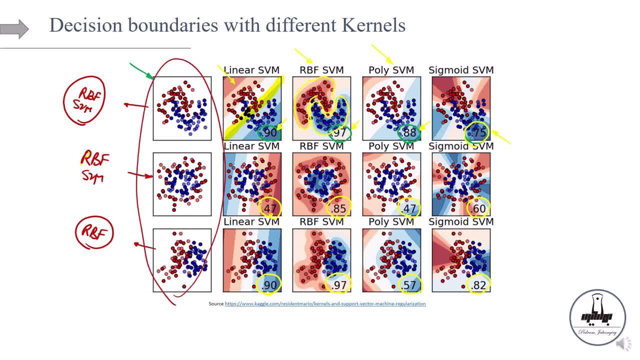 regardless of the shape of the data. rbf is going to be a very good choice to start with, right? it's a very powerful kernel trick which is going to do a decent job, especially when the dimension of the data is very large, right? so rbf is going to reduce the dimensionality by the by, basically, 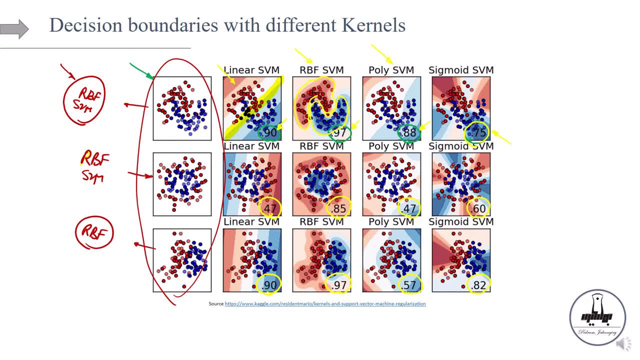 forcing the coefficients in higher dimension towards zero. so this, this is also on top of, and the uh, the other, the existing powers of any kind of kernel trick, right? so maybe it's a good idea to always start with the rbf and then try other and try other, the. 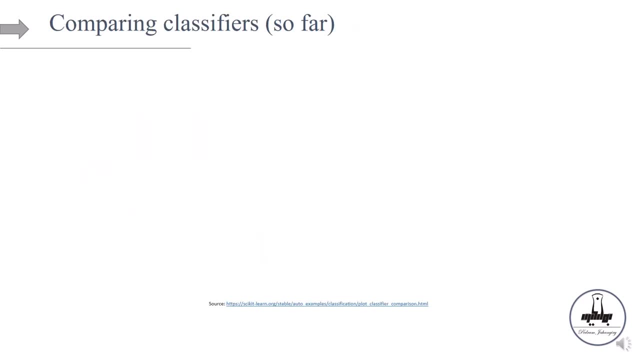 basically kernels down the road. okay, so let's wrap up this episode by going over some exercise together. we're going to compare the classifiers that we have learned so far in this course, right? so imagine the data set is this one and i want you to think of three classifiers, right? 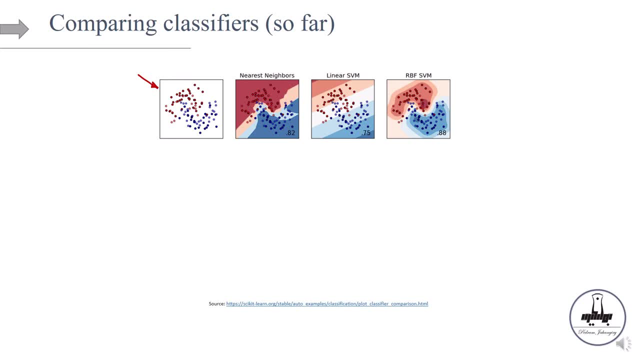 so k? nearest neighbors, linear svm and rbfsvm, right? so this? here we have knn, linear svm and rbfsvm. so if the data is something like this, we know that rbfsvm is going to do a very good job and here knn is also very powerful, right? so what if we talked about knn in the previous episodes? 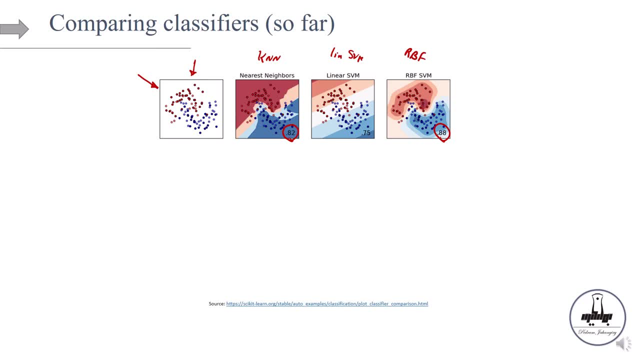 right and when the dimension of the data is small. so in this case the dimension of the data is the standard linear svm and rbfsvm, right, so the data is so like. it's basically two different things. so the dimensionality of the data is only two. KNN is very simple, yet powerful model, and we are seeing. 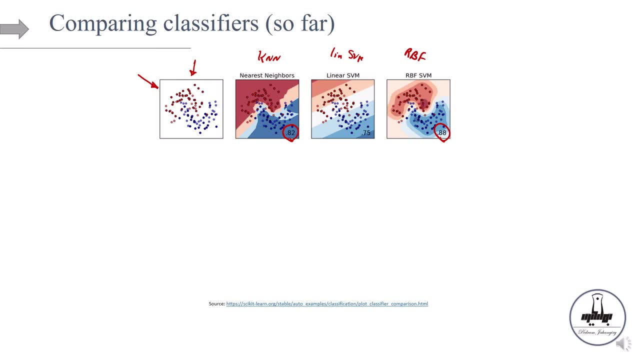 the performance right. It's beautifully capturing the non-linearity in the data, the non-linear pattern existing in the data. okay, So linear SVM is going to do the worst job among these two models. Now for the next data set. I want you to pause the video and come up with the answer on. 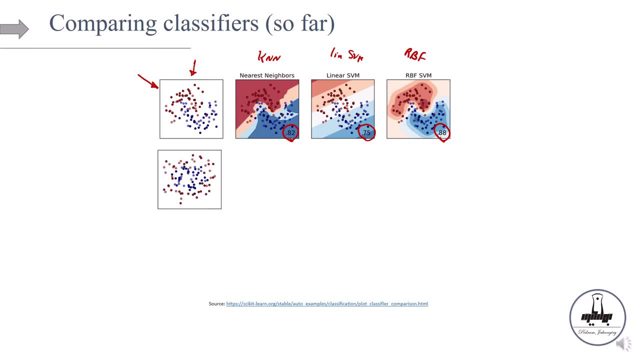 your own. okay, So imagine this is the data set- Which model is going to be the winner: KNN, linear, SVM or RBF? I hope you got the right answer right. So the winner is going to be RBF. 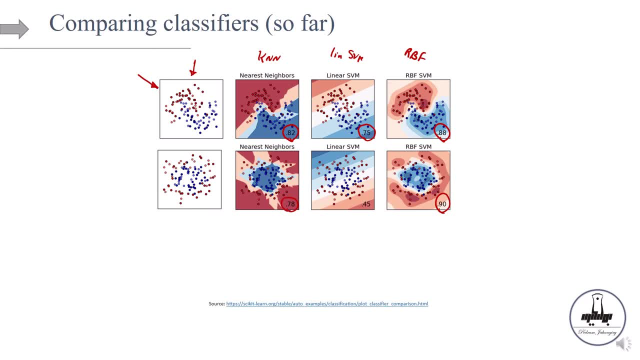 SVM, but again, not surprisingly, KNN is going to do a good job because the dimensionality of the data set is small and KNN is able to perfectly find these closer neighborhoods, right And linear. SVM is going to do the worst job because the data set is non-linear receivable. Finally, what about? 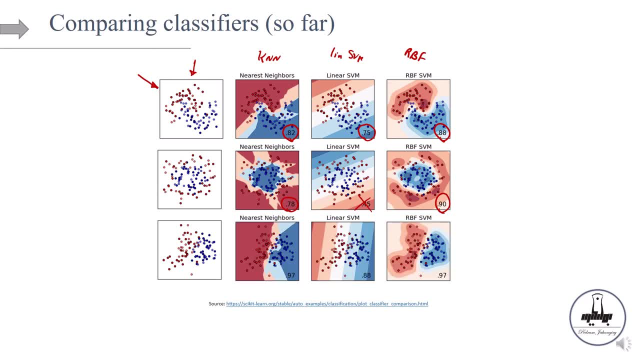 this one. So what's your guess? Yeah, I hope that you're on the right track. So all of the models are going to do a relatively decent job when the data set is linearly separable, right, And yet again, RBF is going to be one of the best performers. So, when the data set is linearly, 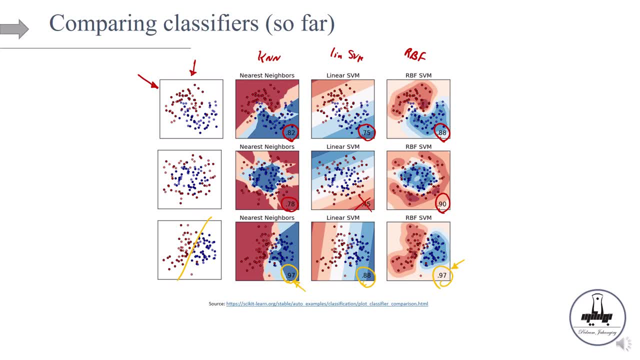 separable KNN is also performing well. but be careful: KNN is powerful only when the dimension of the data set is small right, And because of that curse of dimensionality, KNN is going to suffer a lot when we go to higher dimensions. However, RBF is able to handle those high.